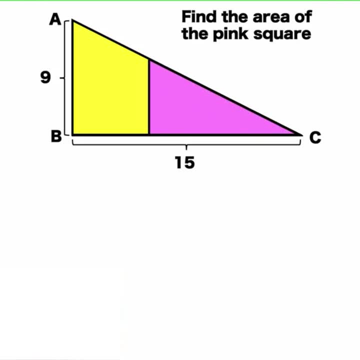 and let's identify this other right triangle. Let's insert again our pink square and call this side as side DE. We know that the length of the side of this square is A units. That means side BE is also A units and since the length of side BC is 15 units, then the length of side EC must be. 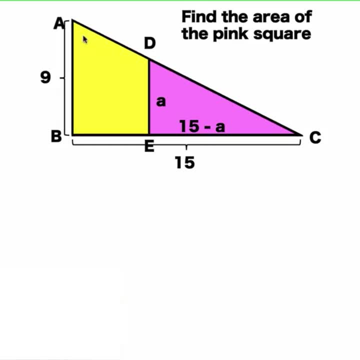 15 minus A units. Now let's concentrate on these two parallel lines. We know that line AB and line DE are parallel because we have a square previously here, And since these two parallel lines are cut by transversal AC, then if you let the measure of angle BAC. 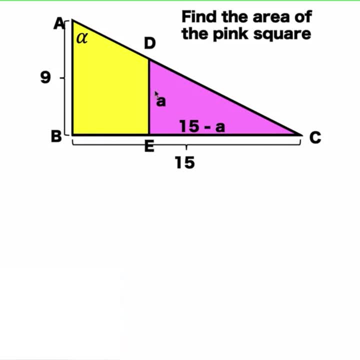 to be equal to alpha, then the measure of angle EDC must also be alpha, because corresponding angles on the same side of the transversal are equal. Now let's assign a value of beta for the measure of angle DCE. Then let's detach these triangles so we can analyze them better. So we have here: 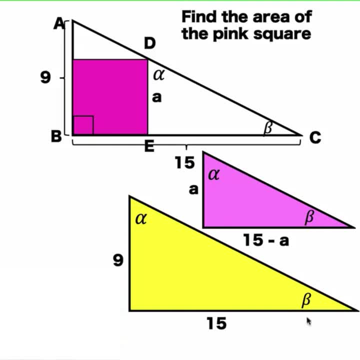 two right triangles. Their two corresponding angles are congruent. It follows by the angle angle similarity that the angle angle is equal to the angle of the transversal. So we have here two triangles. The yellow and the pink triangles are similar triangles And since they are similar, 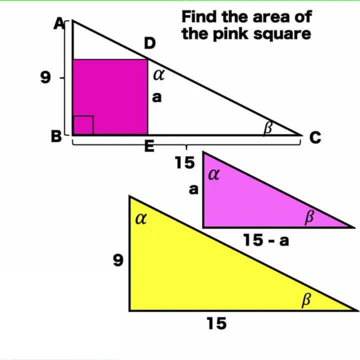 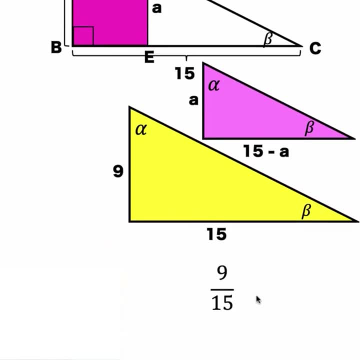 triangles. their corresponding sides are proportional, And so we can now form this equation: This side over this side is 9 over 15.. That is proportional to this side measuring A units over this side, measuring 15 minus A units. Then let's perform the computation. 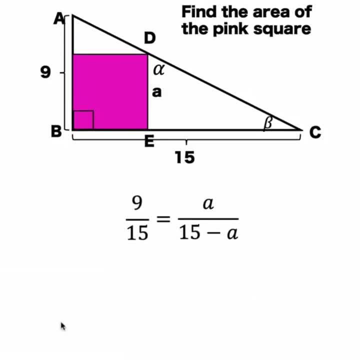 We multiply both sides of the equation by the least common denominator of 15 times the quantity 15 minus A And, simplifying, we can cancel out these 15 and 15, so the left side is 9 times 15 minus A. At the right side, this factor 15 minus A, divided by this denominator. 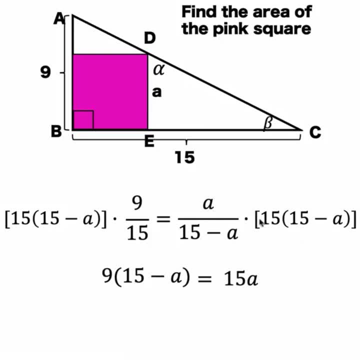 15 minus A is equal to 1.. So what is left is A times 15, which is 15A. Then let's distribute 9 to the quantity 15 minus A to get 135 minus 9A, and copy the right side and add 9A to both side of the.